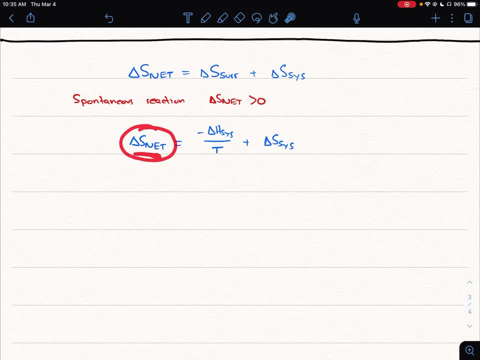 what this term is. You know, what is this change in entropy of the universe? That's a very difficult thing to determine, And so what chemists have done is they've taken this equation and we've defined a new term, And so I'm going to show you how algebraically we got there, And so I'm going to start off. 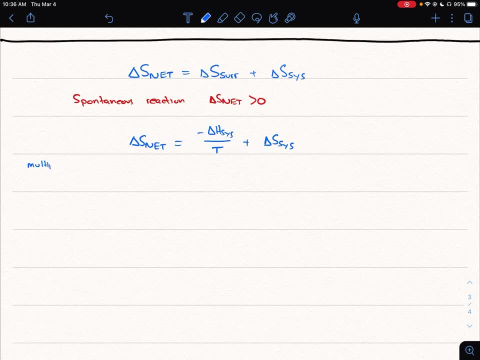 and I'm going to multiply everything by negative T. Okay, so we're going to multiply everything by T- negative T, And so we get negative T. delta S net equals T delta S net, And so we're going to multiply everything by T- negative T, And so we get negative T delta S net. 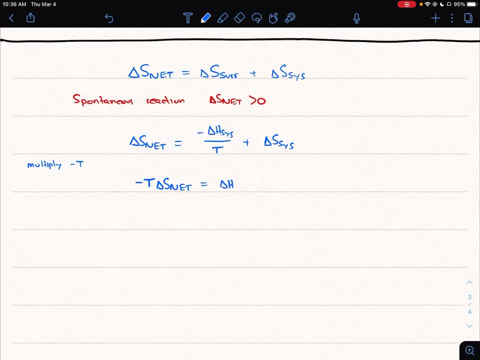 And so we get negative T delta S net, Delta H, Because we've removed that negative and then divided by T And now minus T times delta S of the system. So now we have a term where we have this negative T delta S net is equal to delta H and that's delta H of the system. 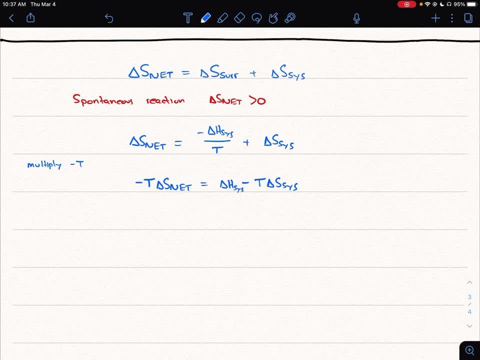 Minus T times delta S of the system. What chemists then did was they defined a new term. So we're going to define a new term And they're going to say that this negative T delta S net is defined to be delta G. 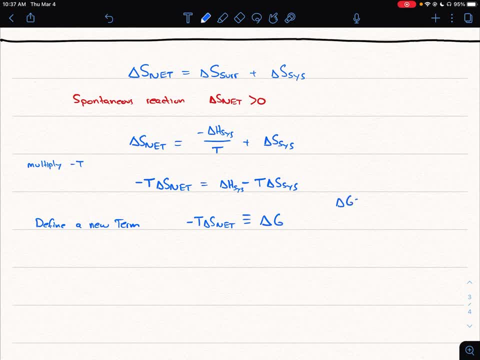 And delta G is what we call Gibbs free energy. And when we look at that and we see this delta G term, we now have an equation where delta G is equal to delta G, Delta H minus T, delta S, And in this equation everything refers to the system. 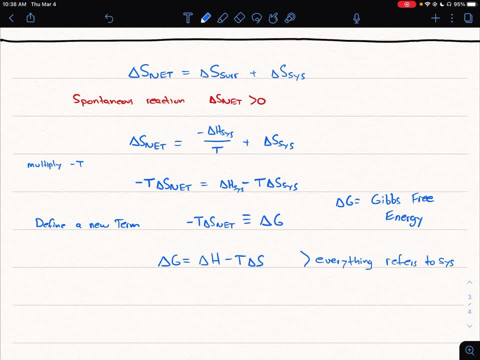 So I dropped the subscript cis from these, because now we have an equation that says everything is of the system And this equation- delta G equals delta H minus T. delta S is probably the single most equation that you will see in general chemistry. 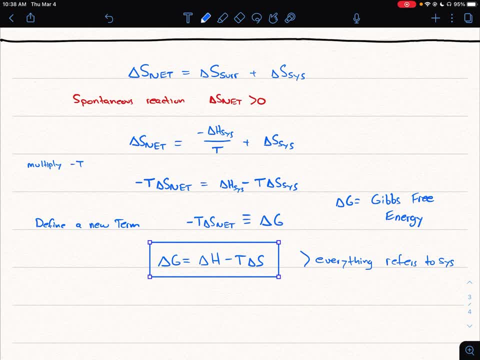 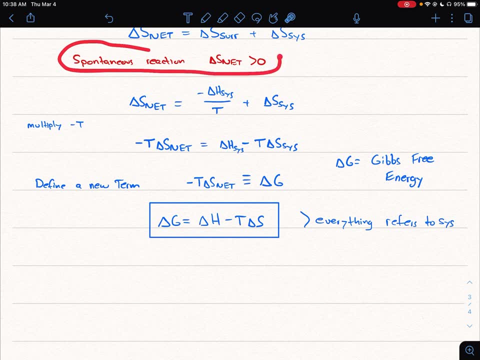 This is our criteria of spontaneity And I want to look at this and just recall. we said a reaction is spontaneous when delta S net is greater than zero. But if you think about our equation down here for delta G, if delta S net is greater than zero, 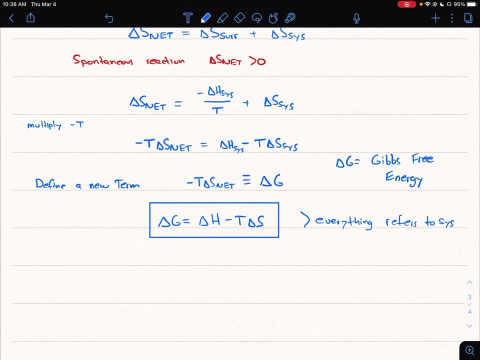 we're going to multiply that by 90%, We're going to multiply that by negative T, And so our reaction is spontaneous when delta G is less than zero, And that's because we have this negative sign here. So if delta G is less than zero, 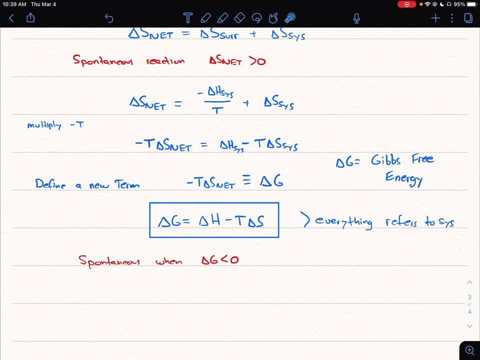 that means that delta S net is greater than zero, And when we think about this equation, the other nice thing what it does is it's a new thermodynamic variable that's put in terms of our delta H and delta S, And so we can think about this. 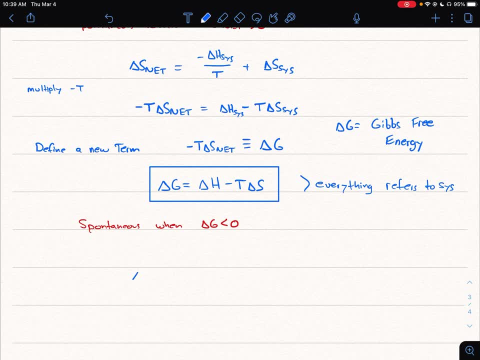 and we can think about our various terms, And so I'm going to write a little table here. We have our delta H, delta S and delta G, And so we can build our table. Those are our terms, And up top we'll say: 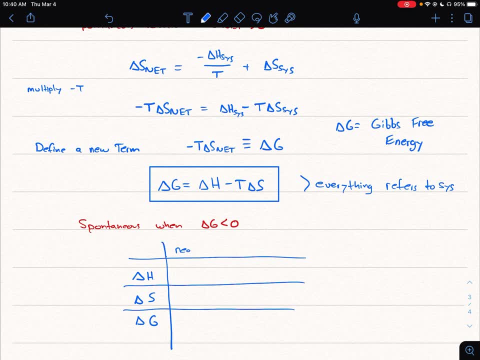 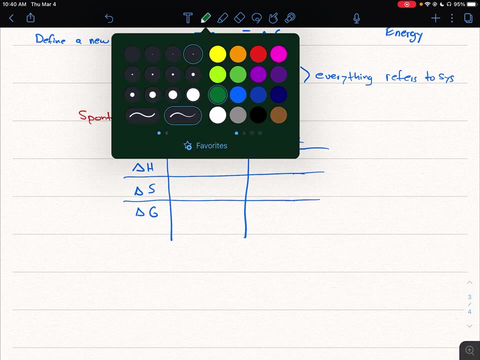 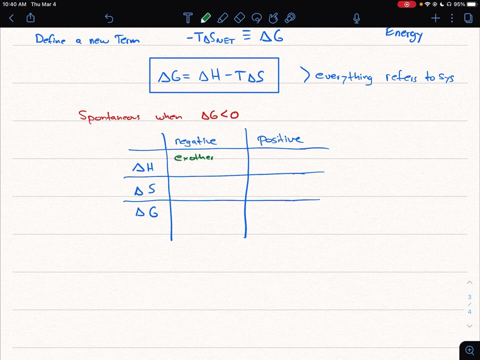 when these terms are negative or when these terms are positive. What does that mean? Okay, And when we think about that, if we think about delta H, if delta H is negative, that means it's an exothermic reaction And that's a favorable process. 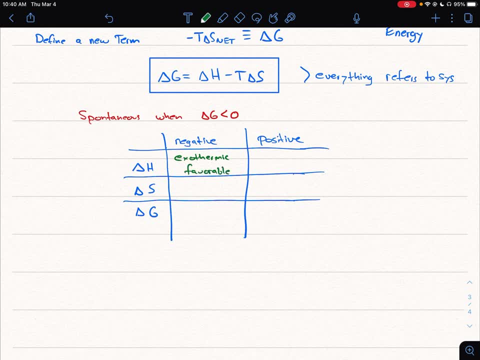 We're going to use the word favorable And when it's a positive delta H, that's an endothermic reaction and that's unfavorable. Now, in terms of our change in entropy of the system. we said when delta S is negative. 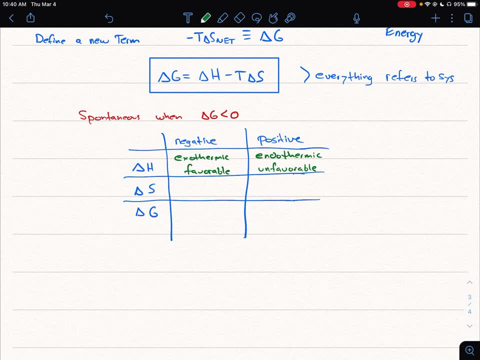 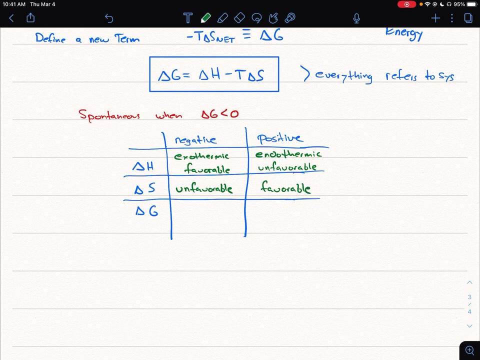 that's an unfavorable. We're losing arrangements. So, when delta S is negative, that's unfavorable, And when delta S is positive, that's favorable. Okay, When it comes to delta G, we're going to say: when delta G is negative. 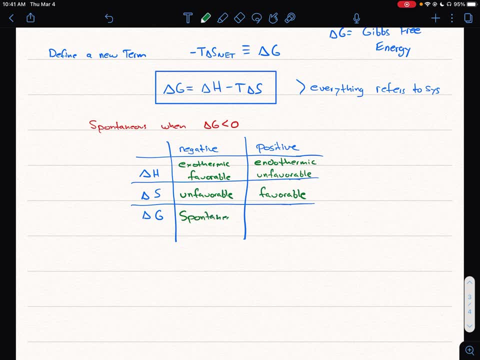 that is our spontaneous reaction, And when delta G is positive, that's our non-spontaneous Yes. And so when we go back to our equation, delta G equals delta H minus T, delta S, we can see we have two terms. 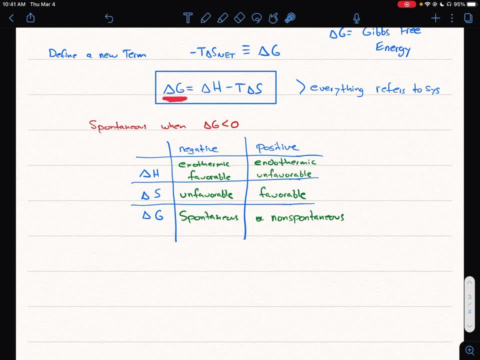 both of which can help make delta G negative and spontaneous. So if delta H is a huge negative number, a very exothermic reaction, that's going to help make delta G negative and spontaneous. By contrast, if delta S is a huge positive, 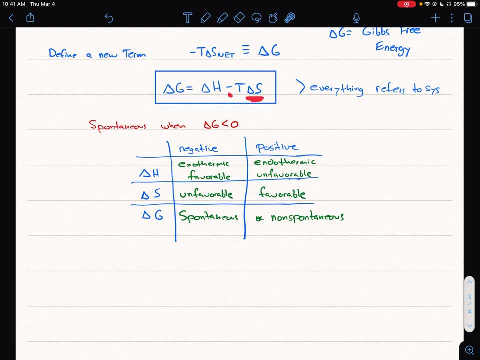 right, then this term, since we're subtracting the positive number, will make delta G negative and that'll be favorable. And so when we think about what makes a process spontaneous, what makes it favorable, it can either be driven by delta H being very exothermic. 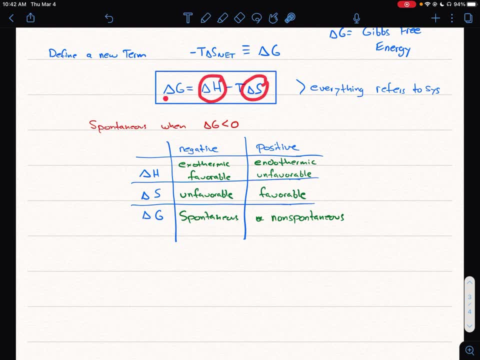 or delta S, being very positive, making this overall negative. In some cases, both are true. We might have an exothermic reaction that also has a huge increase in entropy, and that's a huge increase in entropy, and that's a huge increase in entropy. 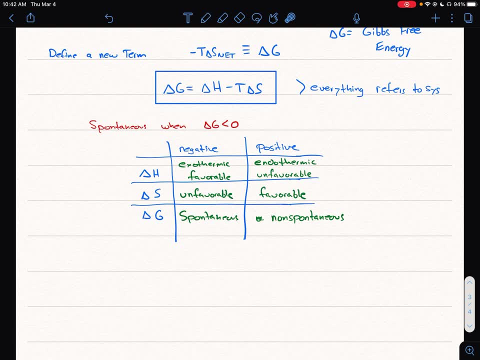 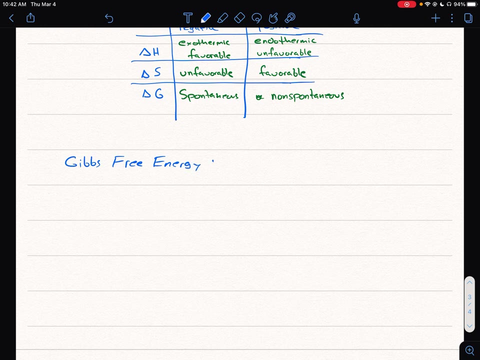 That's a reaction that would be a very spontaneous event Now, when we think about the Gibbs free energy. so Gibbs free energy, right, So that's our delta G. So what do we mean by this free energy? What that really means is: the free energy is really the energy available to do work. 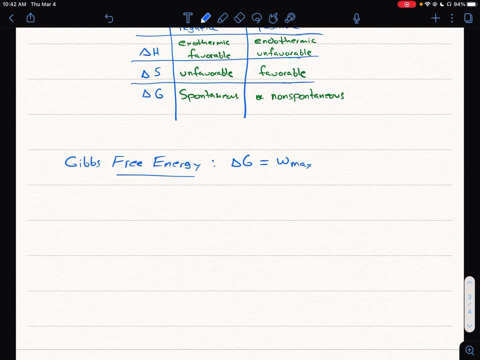 So sometimes you'll see this: the Gibbs free energy is equal to this maximum amount of work. This is the energy available to do stuff. So when we calculate a delta G, that negative delta G that's spontaneous, that negative number that we get, 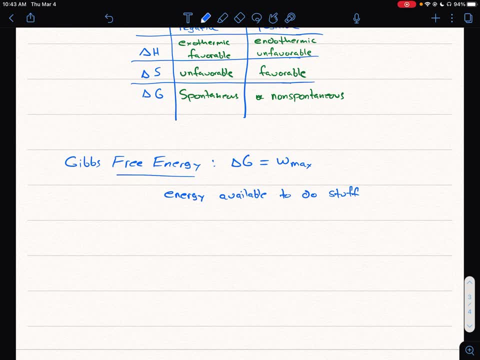 that's the energy we can harness to do something. If it's in our body, it might build a protein, move a muscle. If it's in a car, that's the energy that we can transform into movement. That negative delta G is the energy that is available to do stuff.